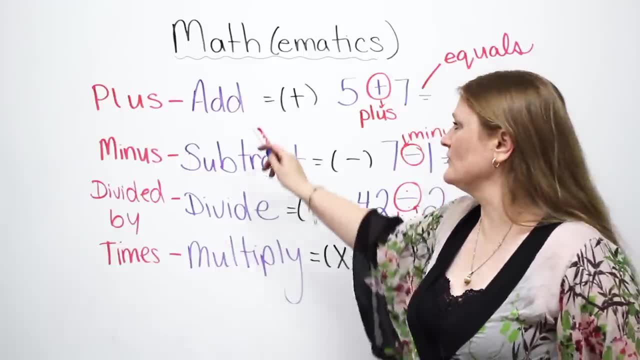 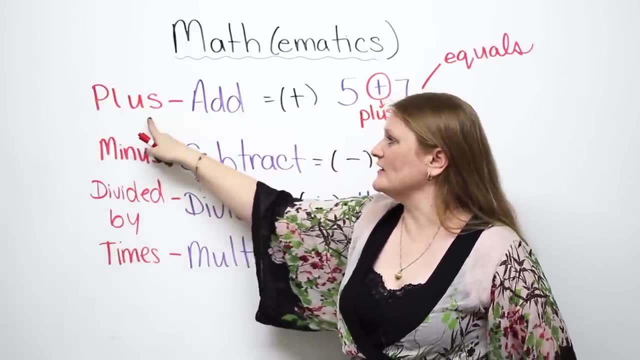 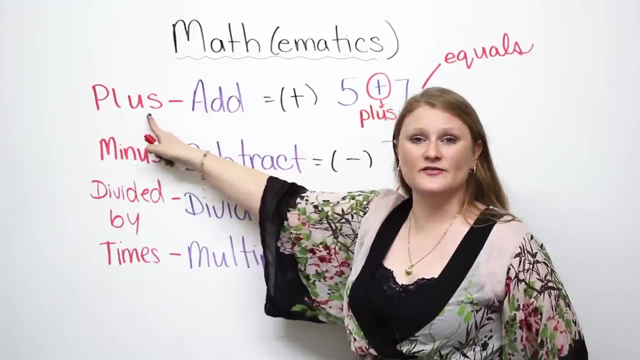 about math in a sentence in English. we don't use these words, We use these red words, So red words. So instead of saying, for example, 5 add 7, we say 5 plus 7.. So if you look at, 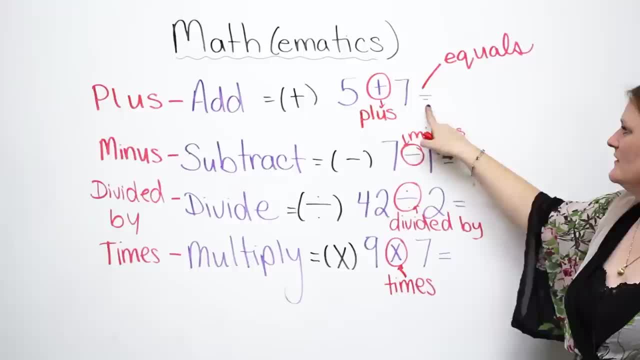 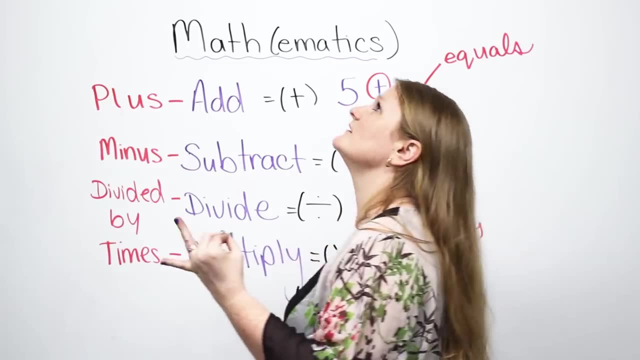 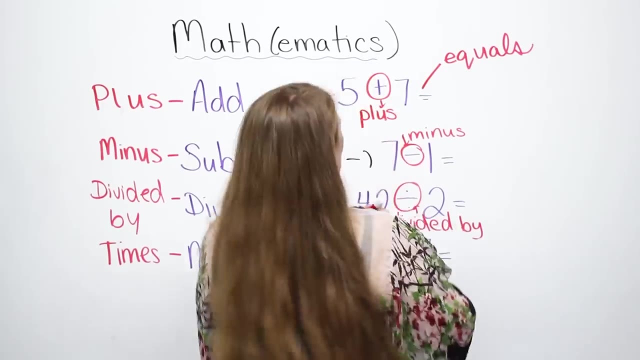 my equation. here we say: 5 plus 7 equals 5 plus 7 equals 12.. I did it, I did it, I did it. I get an answer right. I hope that's right. 5 plus 7 equals 12.. Ding Point for. 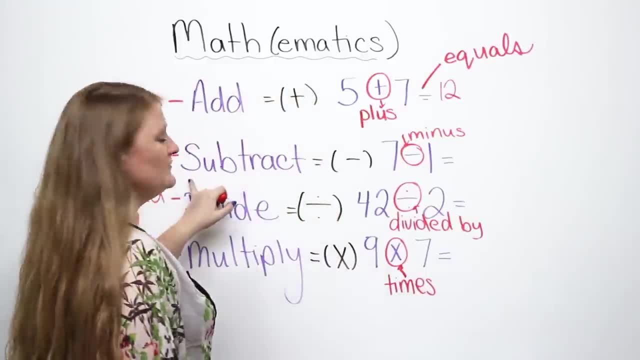 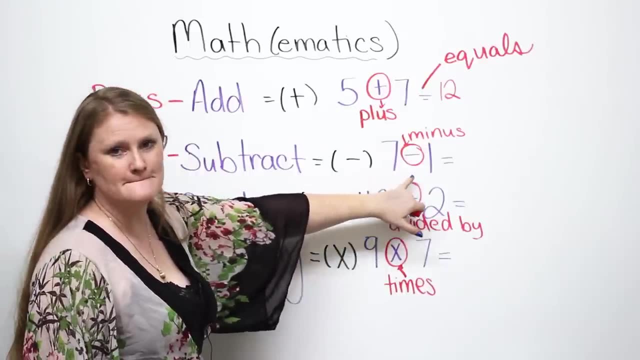 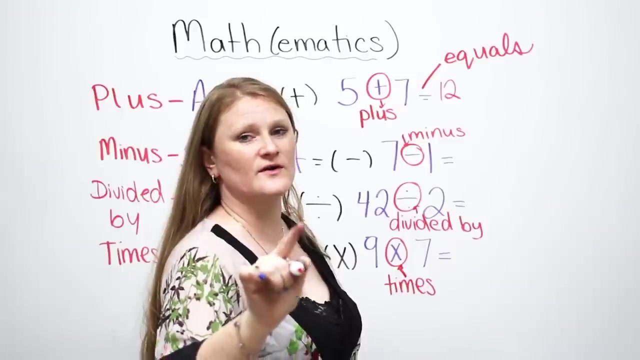 me, The next one's yours. We do not say subtract, We say minus. This is the sign, So we'd say 7 minus 1.. Do you know the answer? If you know the answer, you've got homework Go to. 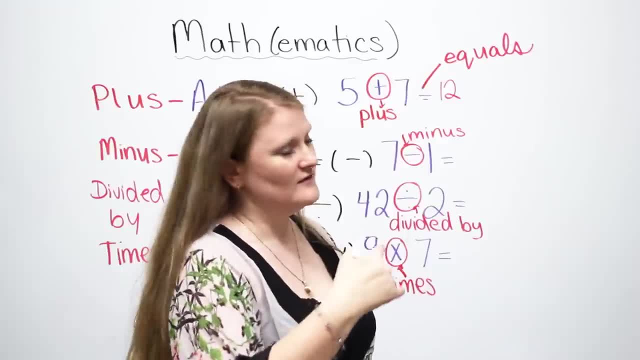 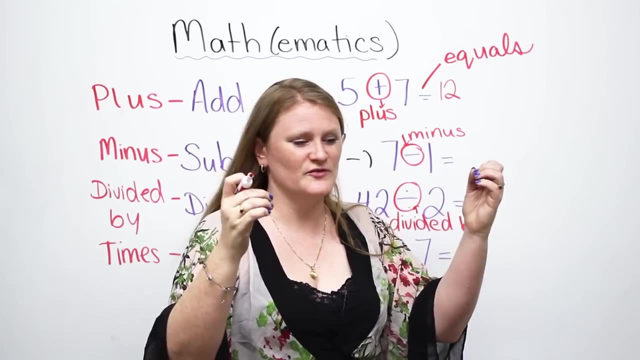 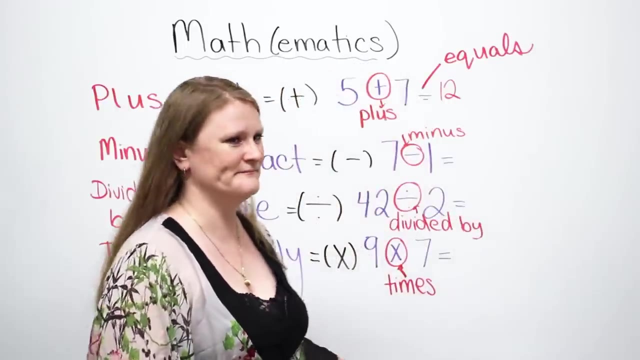 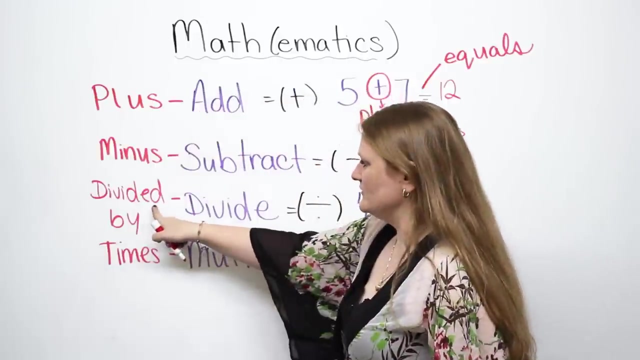 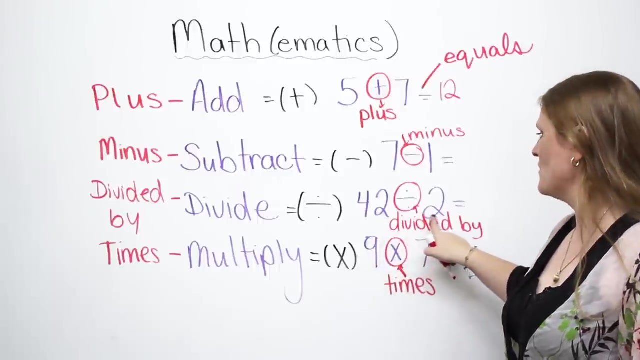 YouTube. Subscribe to my channel. Write the answer to this in the comments You'll win. You'll win amazing prizes like trips to places and money about things. It'll be a fabulous, great time. The next one is divide. This is closer. We say divided by, So we say 42 divided by 2.. 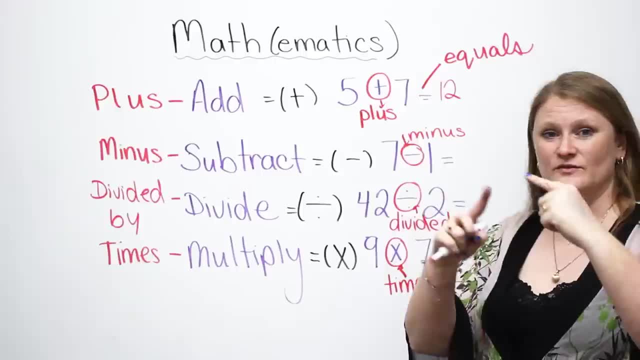 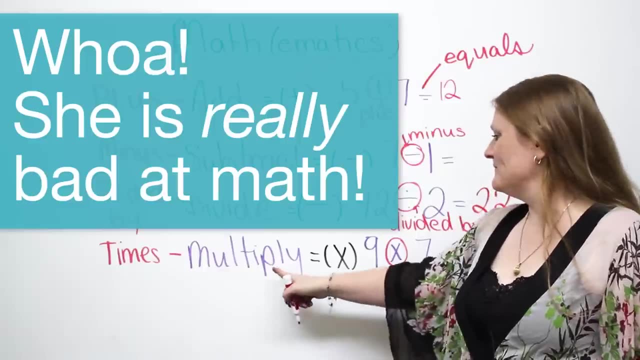 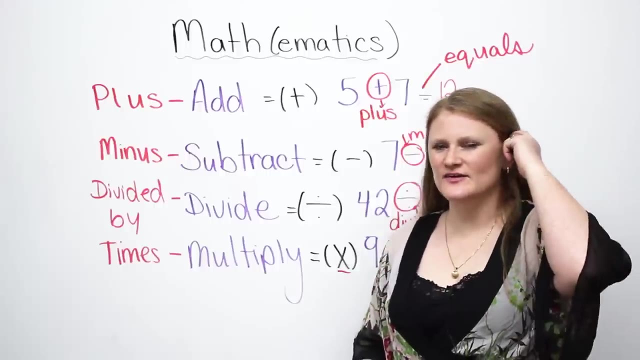 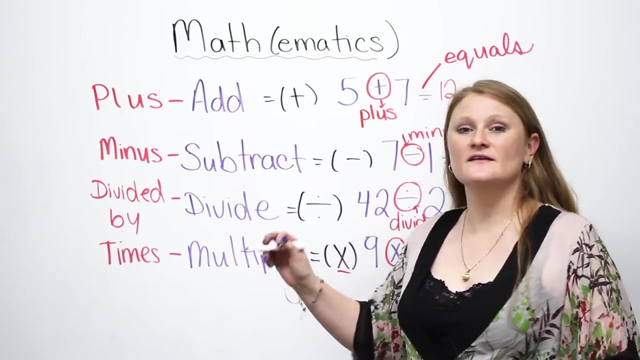 This one's mine, 42 divided by 2 is 22.. The last one is multiply. It looks like a Z or an X. You might say 9x7.. We have to say 9 times 7.. I don't want times as an X Math. 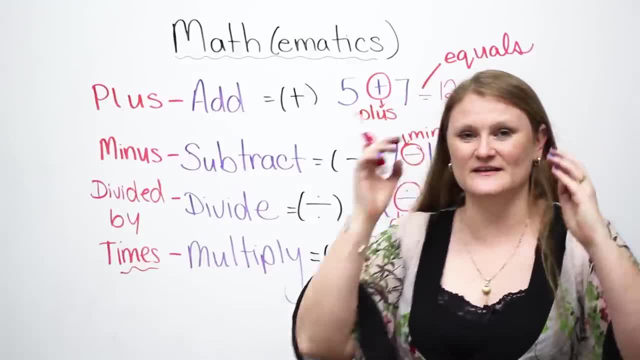 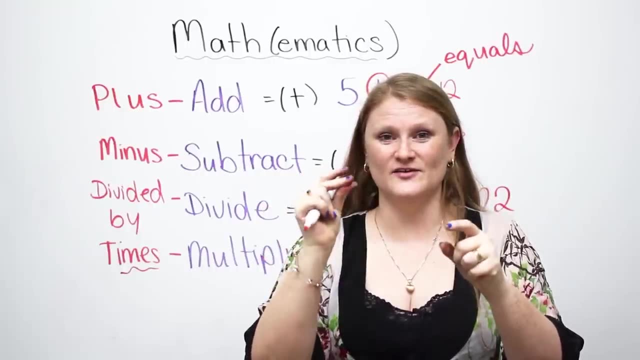 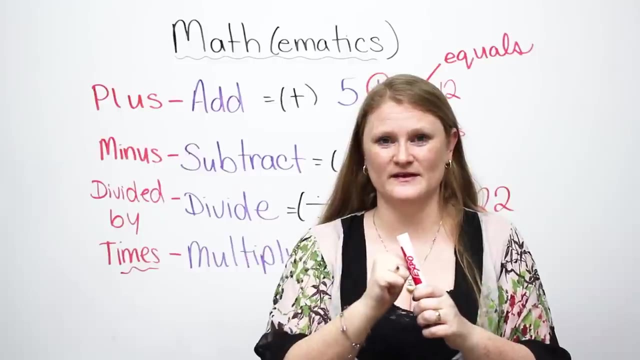 Math is difficult, complicated and hard, but I'm going to teach you a trick. My grade four teacher taught me this. This is the only thing that I can do, like magic for math. If you want to figure out what nine times something is up to ten, you're going to take your fingers and you're. 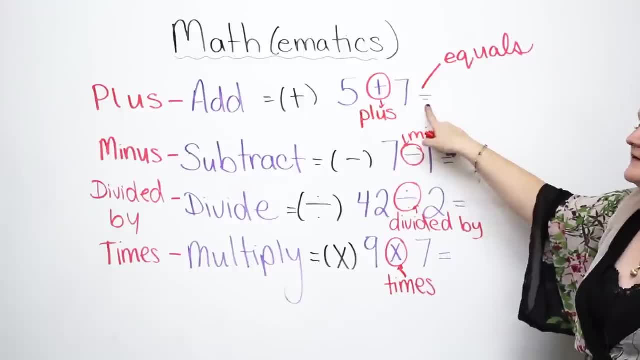 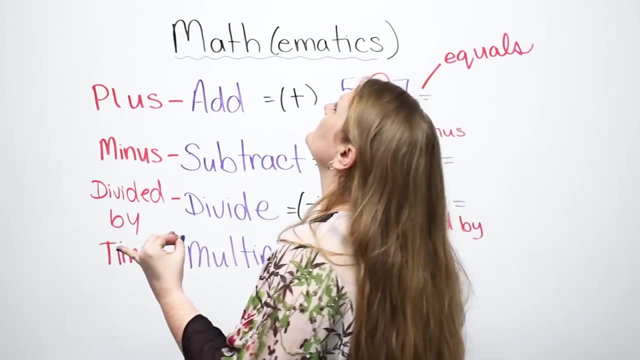 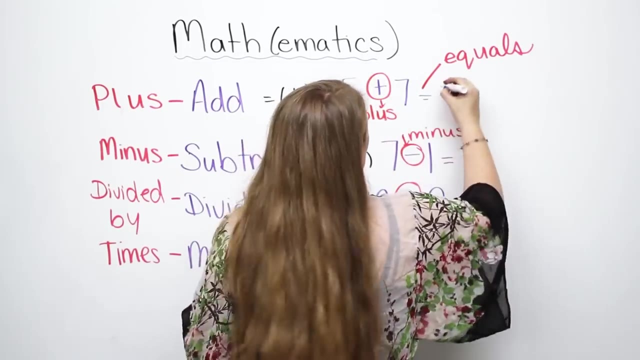 here we say: 5 plus 7 equals, 5 plus 7 equals 12.. I did it, I did it, I did it. I get an answer right. I hope that's right. 5 plus 7 equals 12.. Ding Point for me. The next one's: 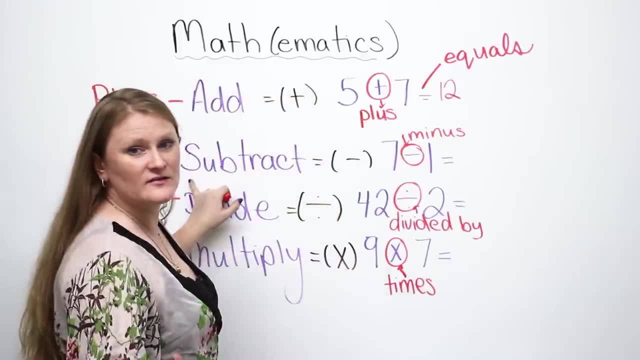 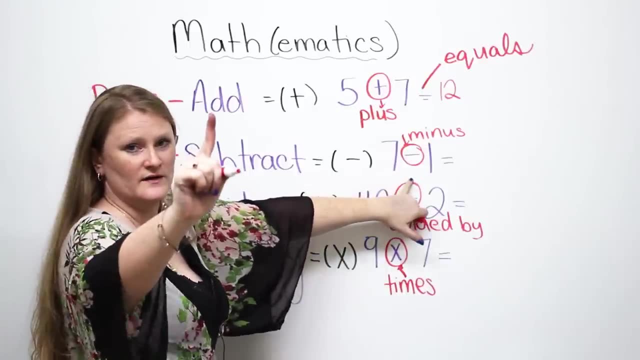 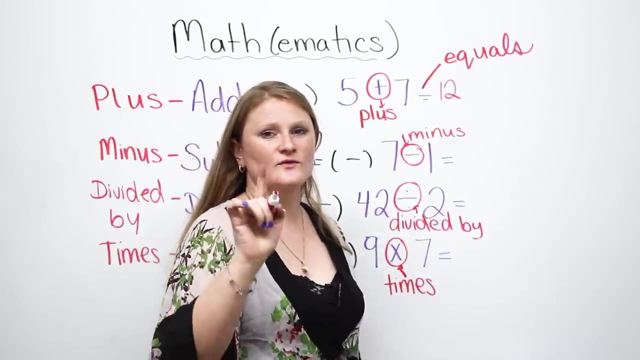 yours. We do not say subtract, We say minus. This is the sign, So we'd say 7 minus 1.. Do you know the answer? If you know the answer, you've got homework- go to YouTube, subscribe to my channel, write. 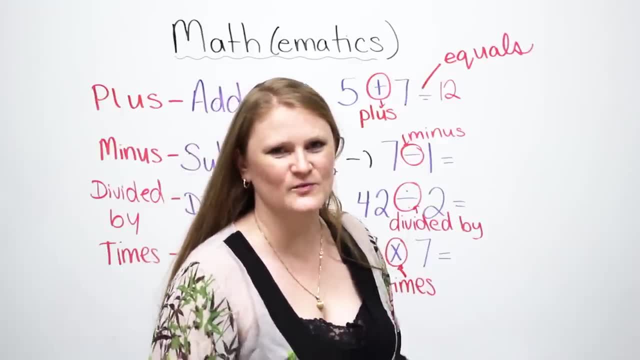 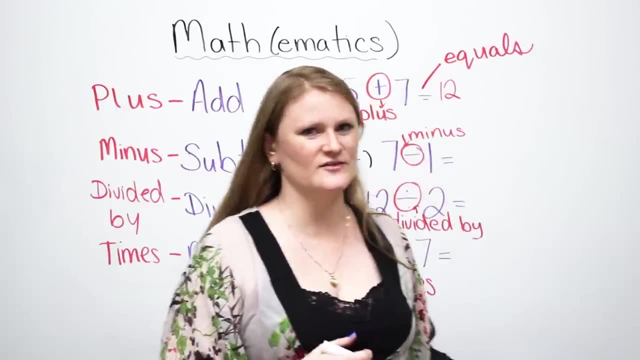 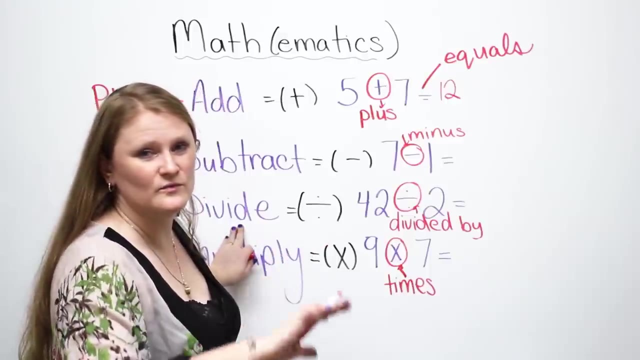 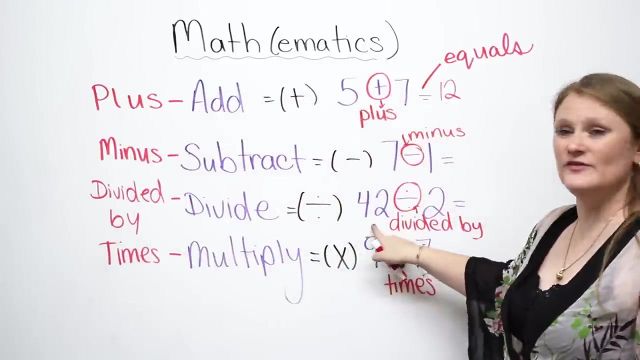 the answer to this in the comments You'll win. You'll win amazing prizes like trips to places and money about things. It'll be a fabulous, great time. The next one is divide. This is closer. We say divided by, So we say 42 divided by 2.. This one's, mine, 42 divided by 2 is 22.. 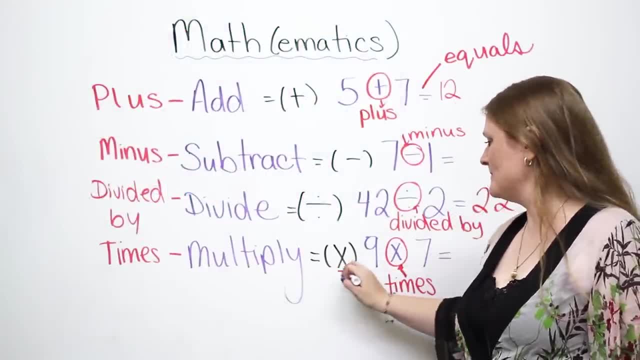 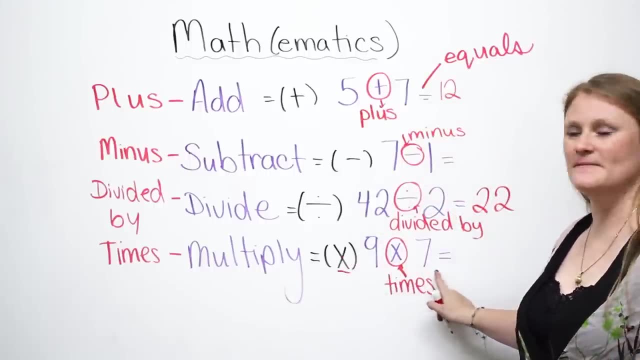 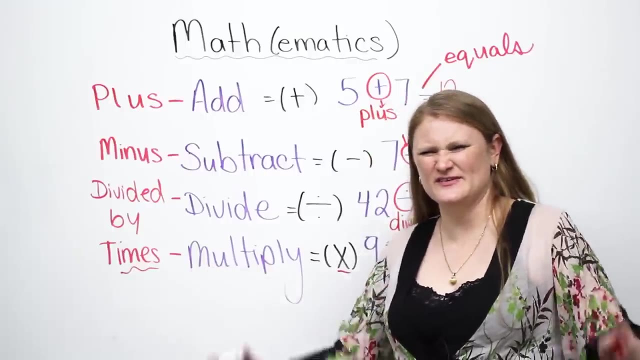 The last one is: multiply. It looks like a Z or an X and you might say, oh, 9X7. Mm-mm, 9X7. Mm-mm. We have to say 9 times 7.. I don't know why times is an X, It's math. Math is difficult. 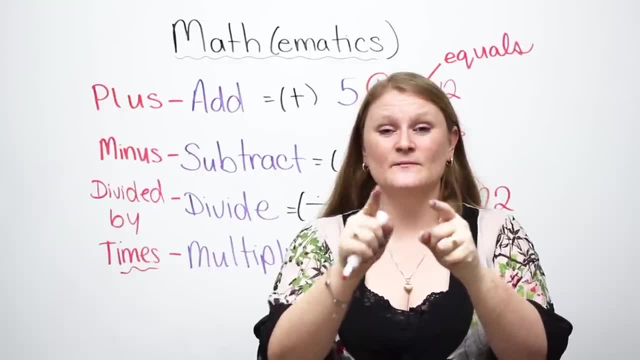 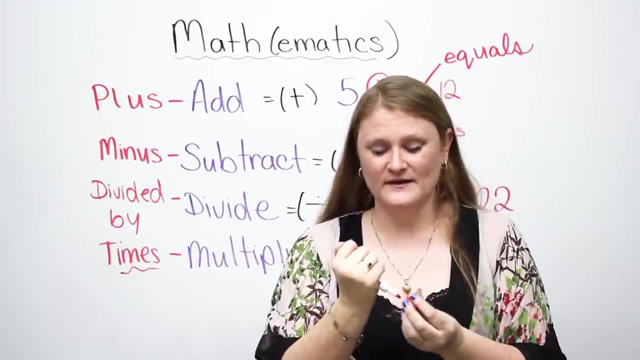 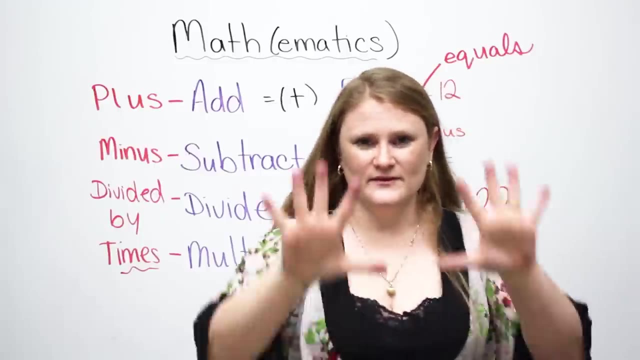 and complicated and hard, But I'm going to teach you a trick. My grade 4 teacher taught me this. This is the only thing that I can do, like magic for math. If you want to figure out what 9 times something is up to 10, you're going to take your fingers and you're going. 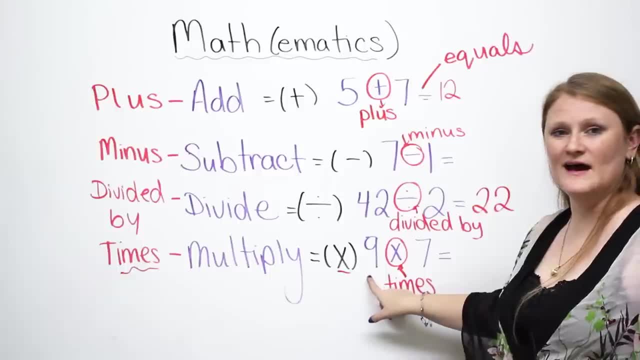 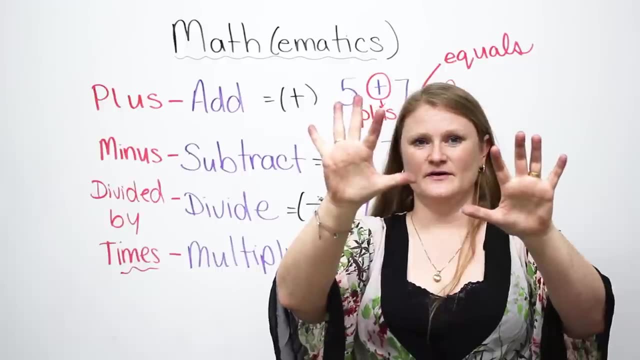 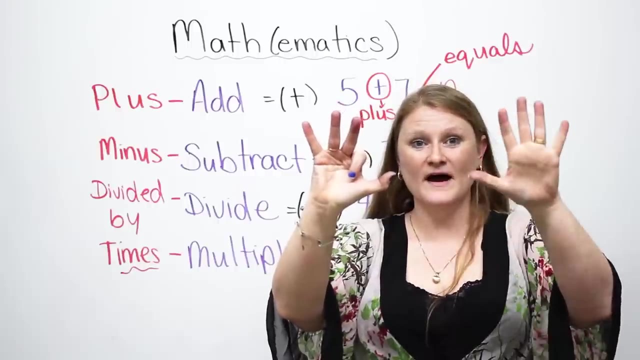 to count. If I want to do 9 times 7, I do this: 1,, 2,, 3,, 4,, 5,, 6,, 7.. And I put number 7 down. I have 1,, 2,, 3,, 4,, 5,, 6 and 3.. Magically, don't change them around. the answer is 63. 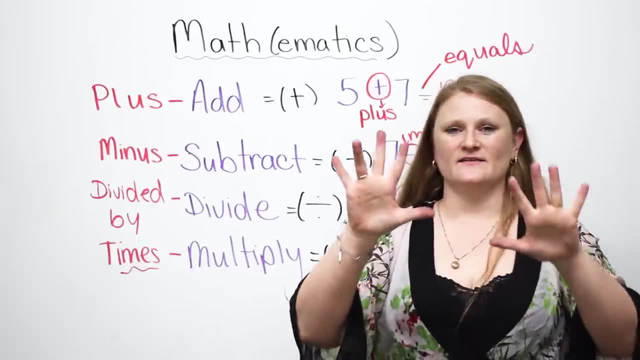 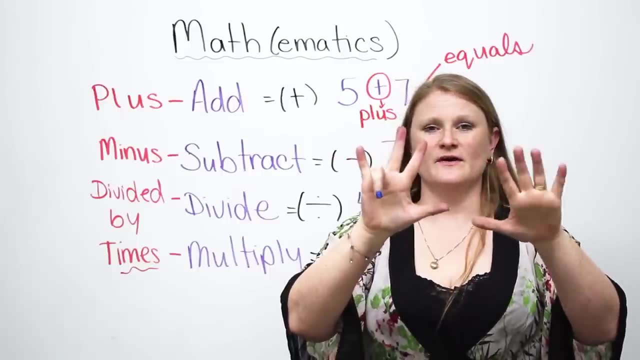 Let's try again: 9 times 9.. So count on your fingers: 1,, 2,, 3,, 4,, 5,, 6, 7.. 1,, 2,, 3,, 4,, 5,, 6,, 7,, 8,, 9.. Put number 9 down. You count how many fingers you have here.